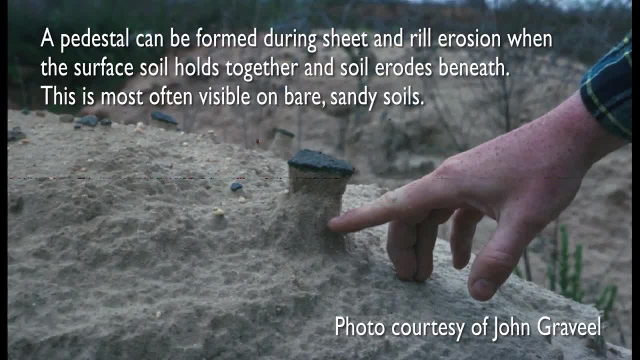 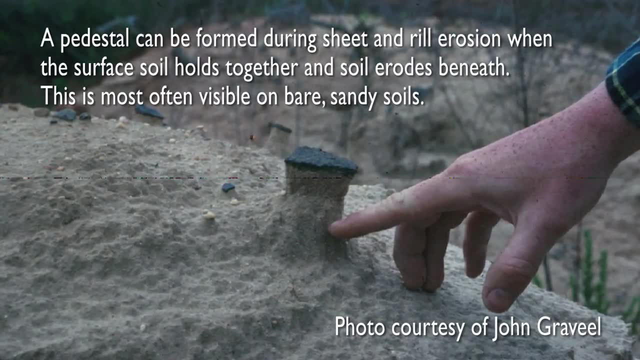 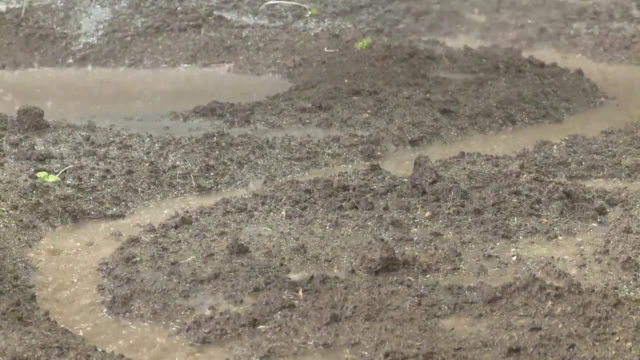 One is called pedestal And pedestal erosion. as the name implies, it's like a pedestal of soil, a pedestal that has a rock sitting on top of it and all the soil has gone around it because of the pounding of the raindrops. The second type of soil erosion that we can 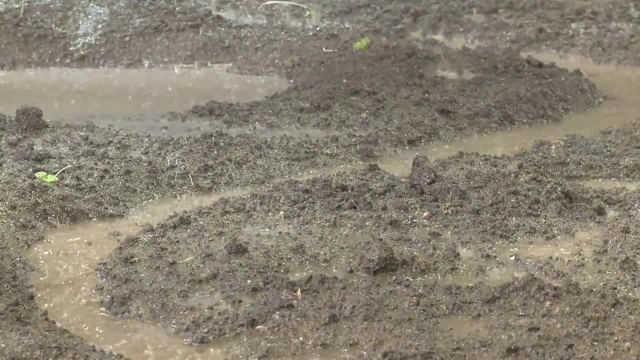 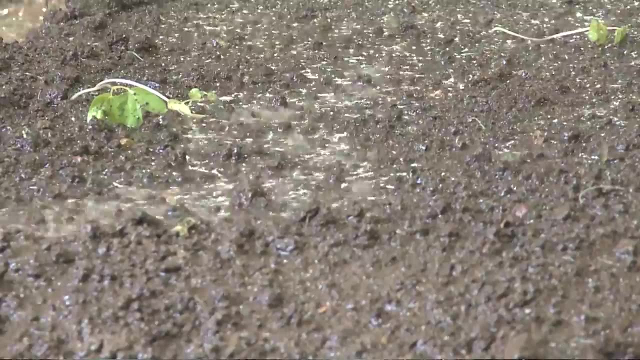 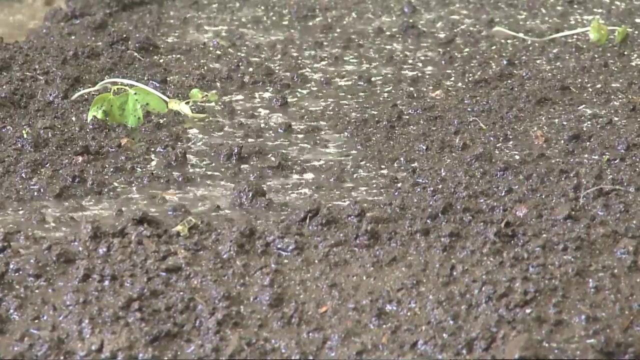 have is real erosion. These are small channels that form in the soil, And these are easily covered up with a tractor. The other type of soil erosion that we have is something that's called sheet erosion, And it's the uniform removal of a thin layer of soil. So 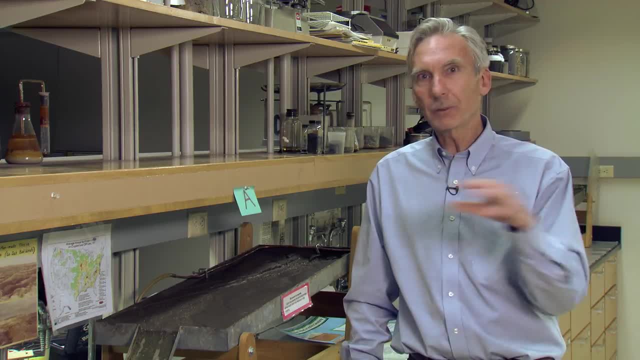 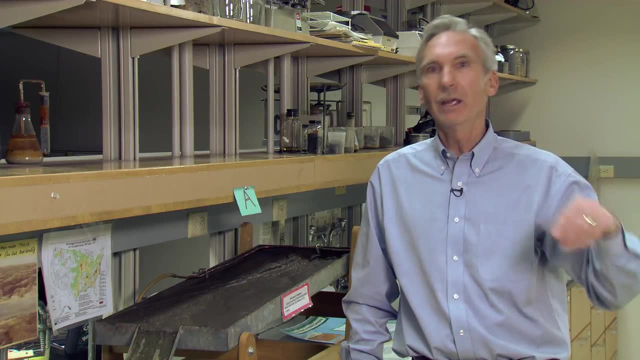 you can't really see this happening. alright, Farmers can't see this happening, But what's happening over a period of time is that you're losing this thin layer of soil every year And what eventually happens is that your productivity goes down and all of a sudden, you realize 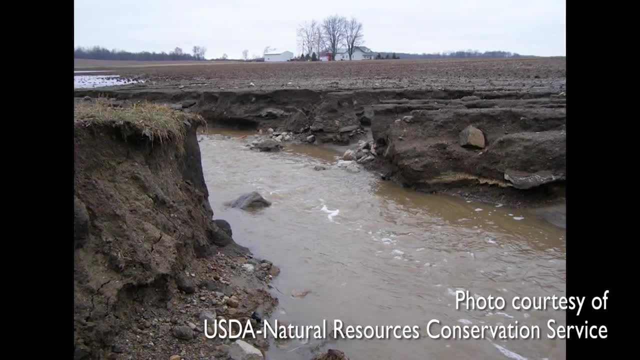 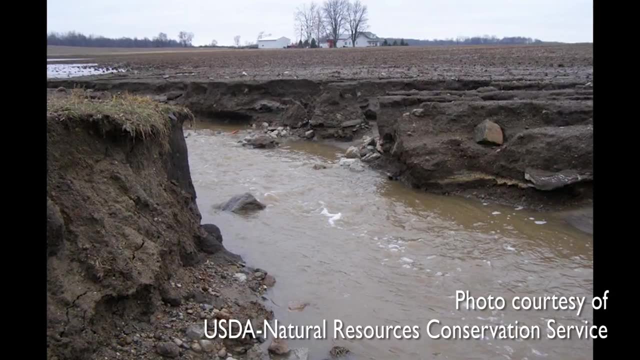 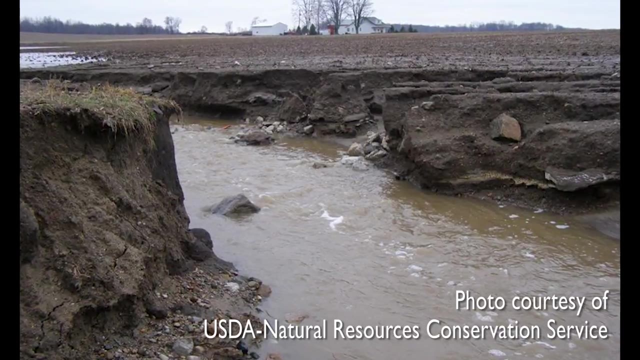 that, oh, I've got a soil erosion problem. The other type of soil erosion that you can have is something called gully erosion, And that's the worst type of erosion that you can have. In gully erosion, essentially what happens there is that these huge changes in 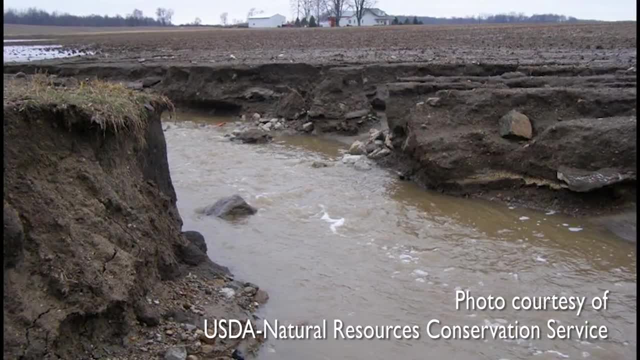 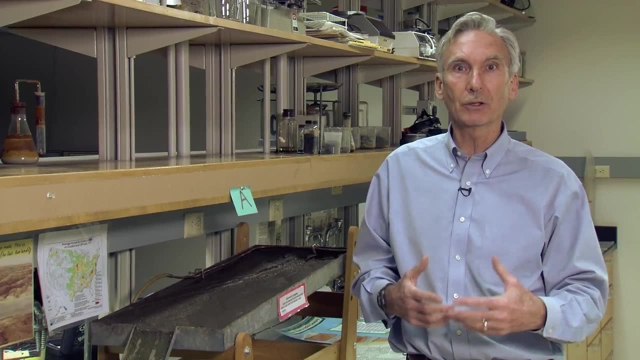 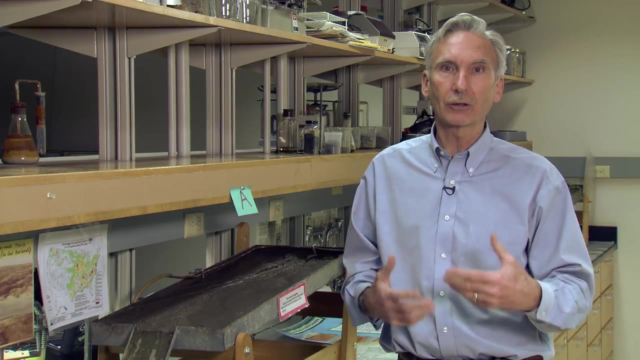 channels form in your soil And what happens is that you cannot cross those with the tillage implement. So what usually happens is you have to come in with some sort of caterpillar tractor to fill in those gullies so that you can carry on traditional agricultural types. 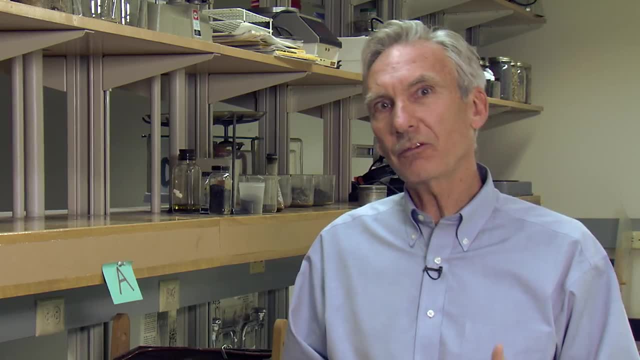 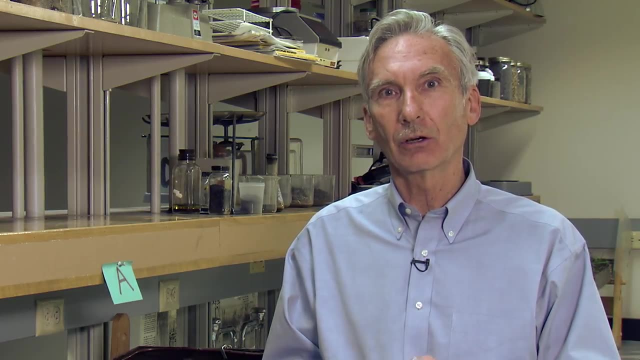 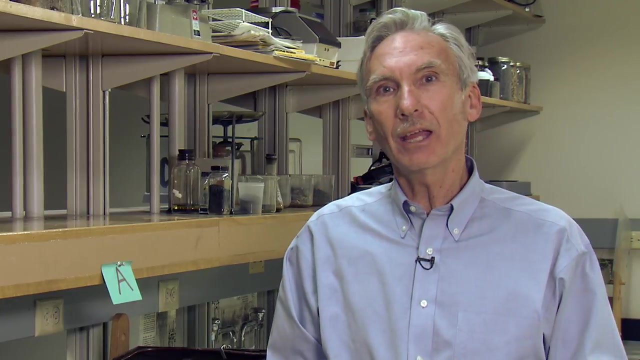 of practices. So the other important fact to remember is that we have two types, major types of soil erosion that can occur Is water erosion, which we're going to spend the majority of our time talking about today, And then we have wind erosion. Wind erosion out in the western part of the United States. 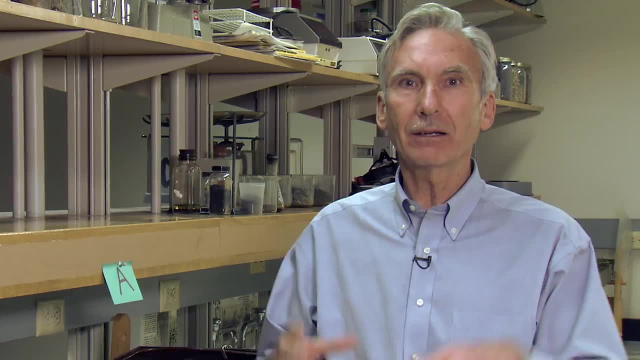 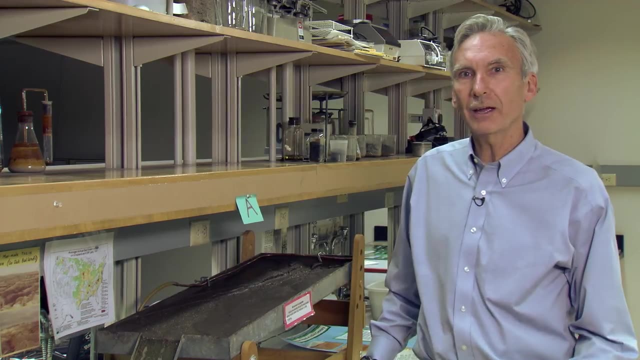 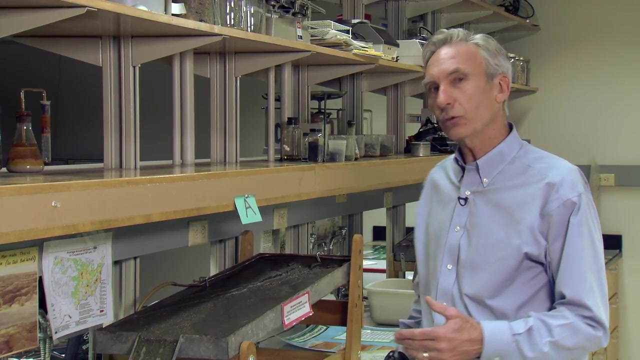 is a big concern Here in Indiana and in the Midwest generally speaking, water erosion is a big concern. So the first type of soil erosion that we're going to look at- again- this is water erosion- is one where we've been tilling the soil year after year after year and not leaving very